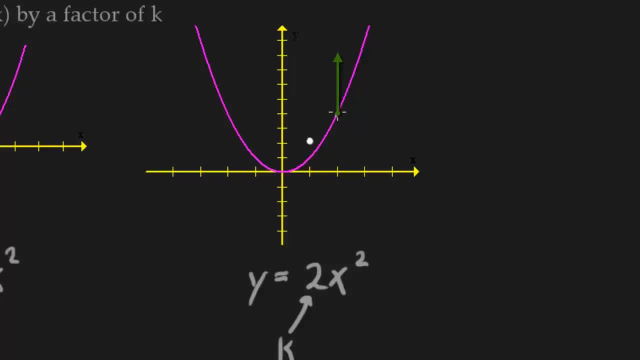 So this is going to go from 2, 4, all the way up to 2, 8,, which would go right here. Now, 0 squared times 2 is still 0, so we get that point Alright. on the other side, it mirrors what we just did. so instead of negative 1, 1,, we're at negative 1, 2.. 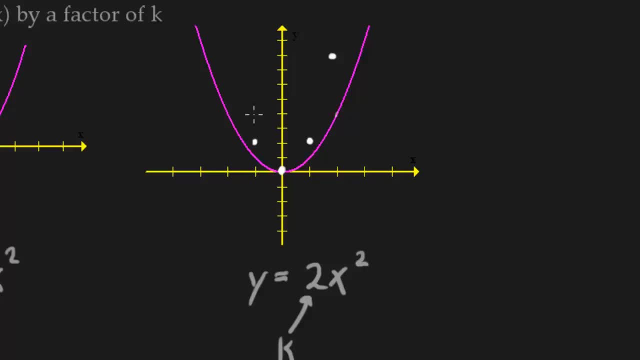 Instead of negative 1, 4,, we're at negative 1, 2.. Instead of negative 1, 4,, we're at negative 1, 8.. Now, if you plug in 3,, 3 squared would be 9, and then we'd have times 2,, which is 18.. 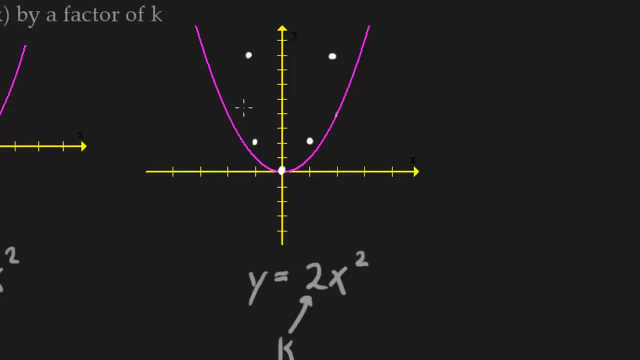 So we wouldn't be high enough. Ooh, I also made a mistake. Alright, negative 2, 8, so that's right there. Alright, so let's connect the dots Now. notice that everything is. it looks like everything is. 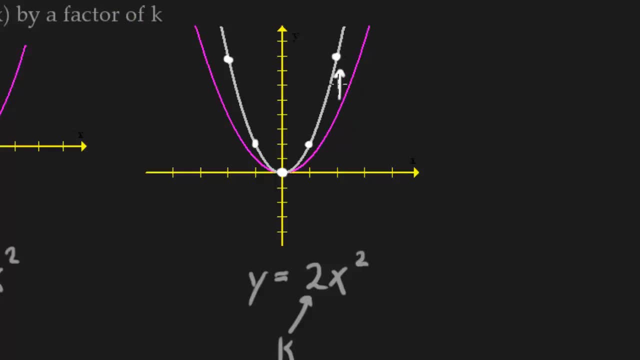 being shifted up, But notice that the shift here is bigger than the shift here. Alright, and that's why it's not actually a vertical shift, because just pretend like you're standing on a rubber band In order to stretch something. something needs to stay fixed. 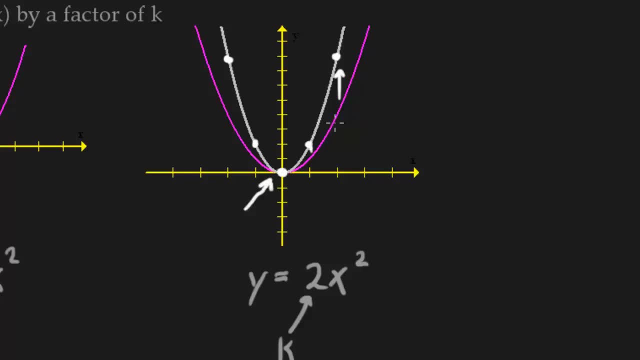 That's our fixed point, in this case the origin. So everything else gets pulled up. As you move farther away from the origin, these changes are going to be larger and larger. But just imagine, you know we have this point here. 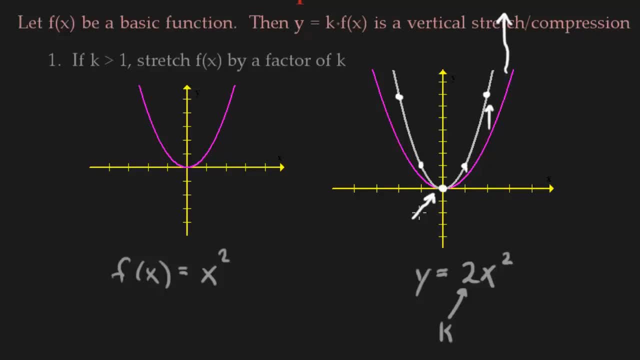 Imagine you're pulling up on a rubber band and that's really what we're doing. So let's see what happens when k is now less than 1.. Now, in this second part, k still has to be positive, but now we're less than 1.. 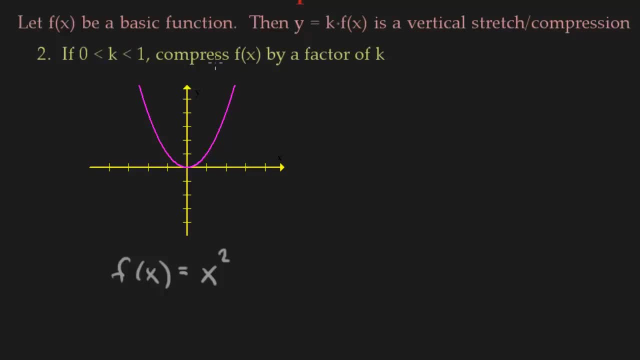 So we're between 0 and 1, and it's going to be a compression, so we're going to compress f by a factor of k. So in the last example we stretched up Now, imagine pushing something down towards the x-axis. 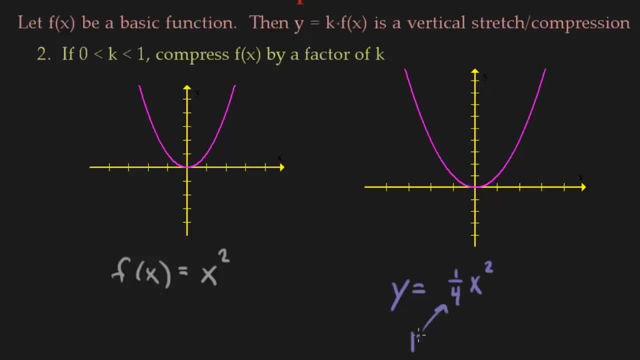 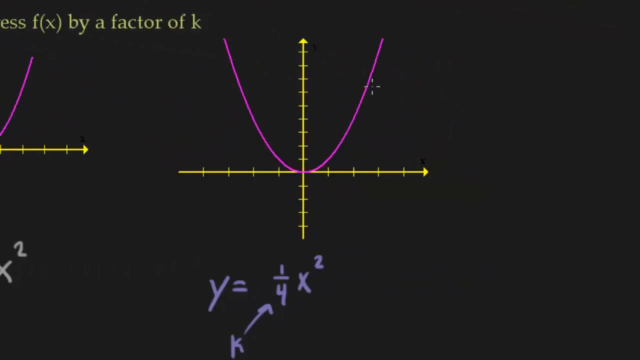 So in this example we have k, which is 1, fourth, which is less than 1, still positive. So what we're going to do is every y-value we get from x squared- because again, this is x squared- we're going to immediately divide by 4..